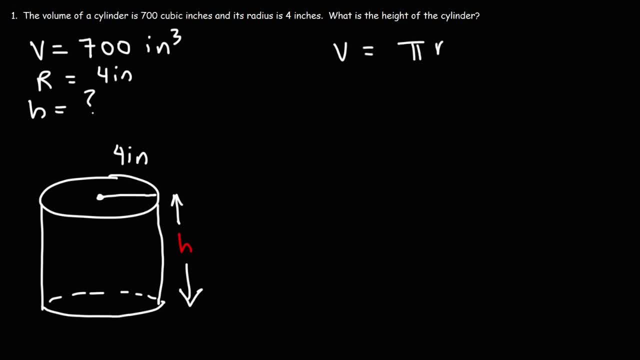 And here it is. The volume is equal to pi. r squared times the height. Now let's plug in what we know. So the volume is 700 cubic inches. This is equal to pi, and then r is 4 inches And we need to square it times h. 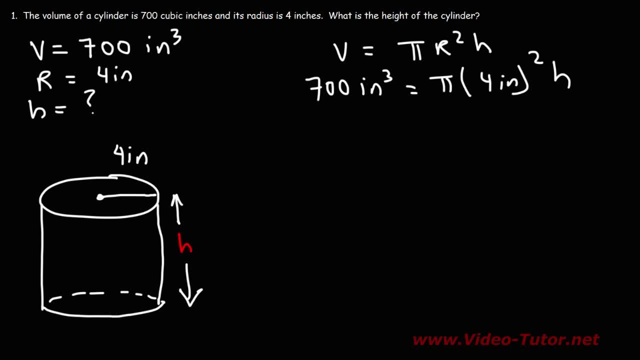 Now pi is 3.14, but I'm going to use the pi value in my calculator, which is 3.141592654.. If you multiply that by 4 squared, that's going to give you 50.. That's a rounded answer. times h. 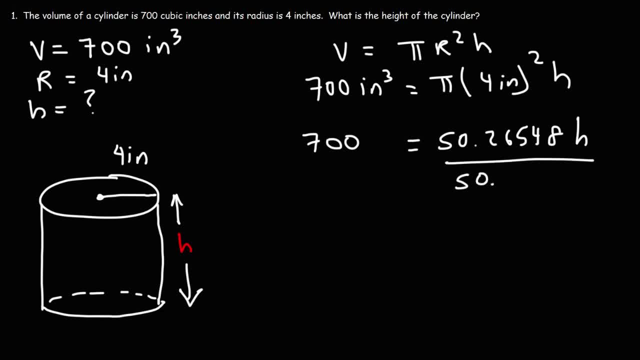 And then to get h by itself, we need to divide both sides by that number. So these two will cancel. and now we're going to get the height of the cylinder. So it's 700 divided by 50.26548. 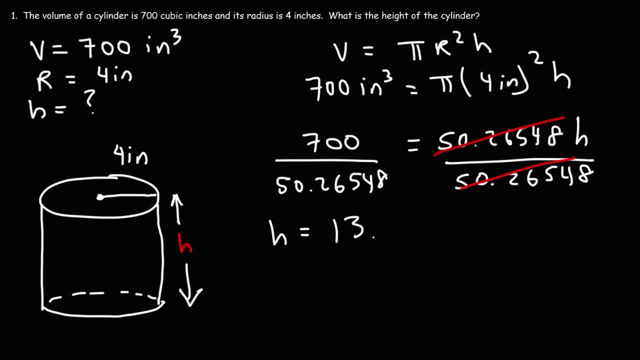 So the height of the cylinder is 13.926.. Now, what are the units? Well, the units is going to be the same as the units for the radius. Make sure these units match. by the way, If they're different, you need to convert one unit into the other. 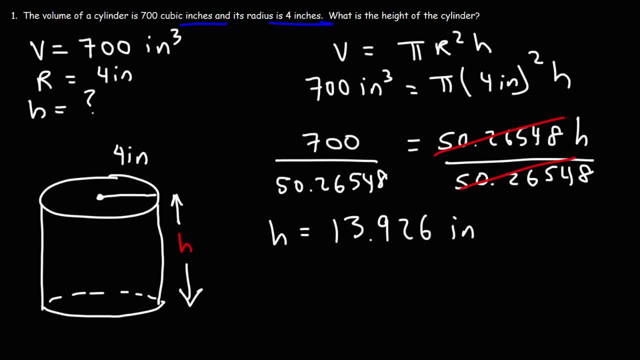 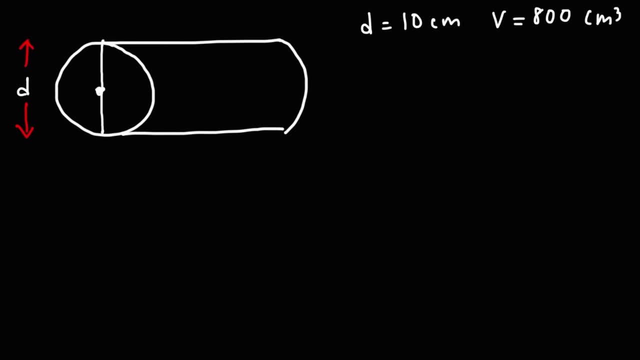 So the height is going to be in inches, So the answer is 13.926 inches. That's the height of this particular cylinder. Now let's work. Let's work on another example problem. So in this problem we're given the volume, like before. 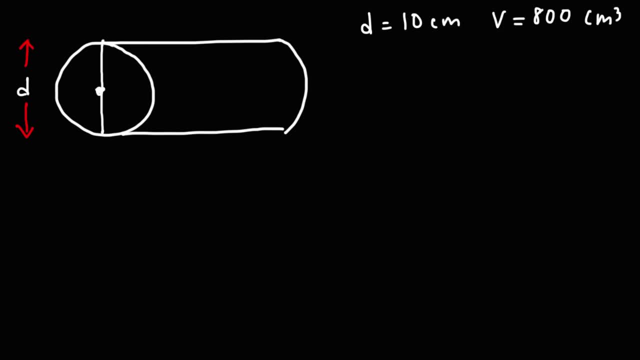 but the difference is it's not in cubic inches, It's in cubic centimeters, And we're given the diameter instead of the radius. With this information, calculate the height of the cylinder, which is the distance between these two extremes. So how can we calculate the height of this particular cylinder? 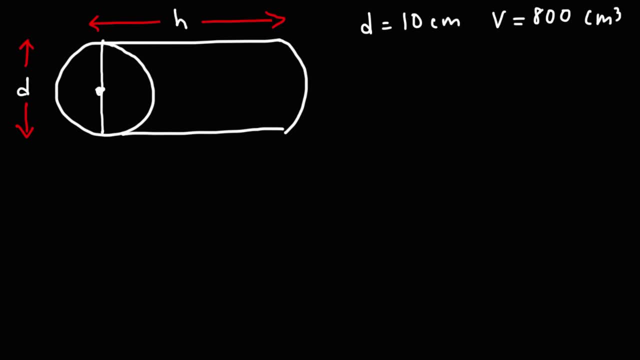 Feel free to pause the video if you want to try this problem. Well, first we need to calculate the radius. The radius is half of the diameter. So if the diameter is 5 centimeters, the radius is going to be. I mean, if the diameter is 10 centimeters, the radius is going to be half of that.